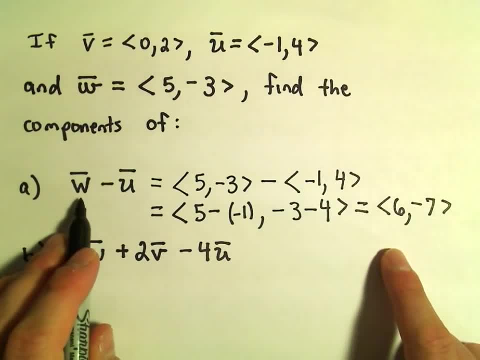 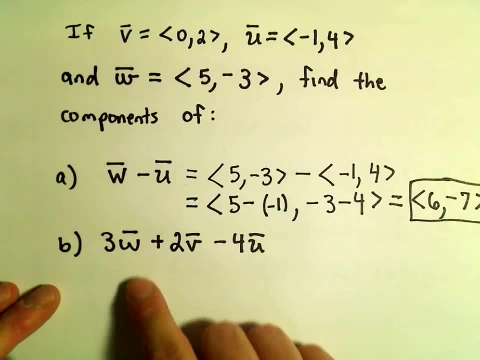 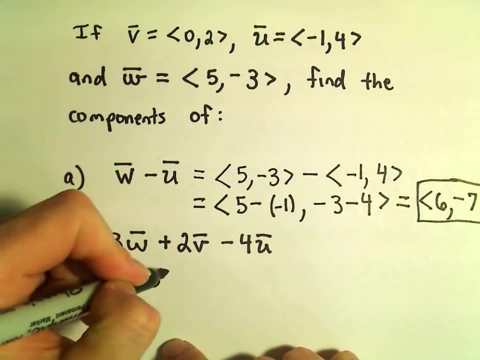 So those would be the components of the vector W minus U. Okay, so part B, kind of combining both ideas. So it says: take 3 times vector W, which has components of 5 and negative 3,, plus 2 times vector V, which has components 0 and 2,. 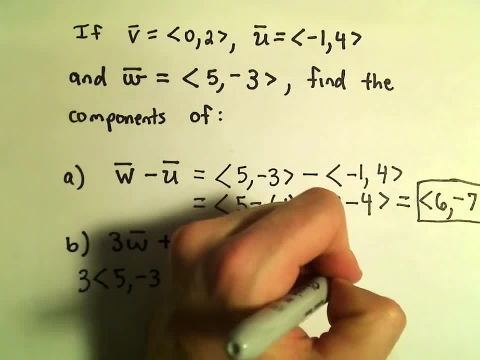 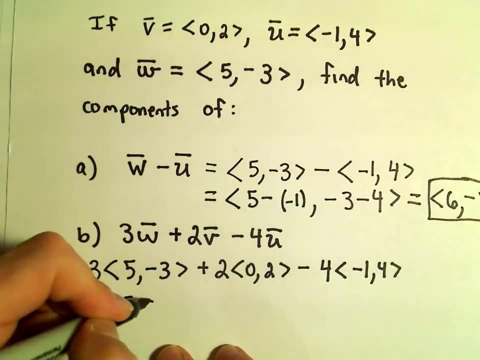 minus 4 times vector U, which has components negative 1 and 2, plus negative 4.. Well, if we distribute the 3, we'll get 15 and negative 9 for the components of our first vector here after multiplying. 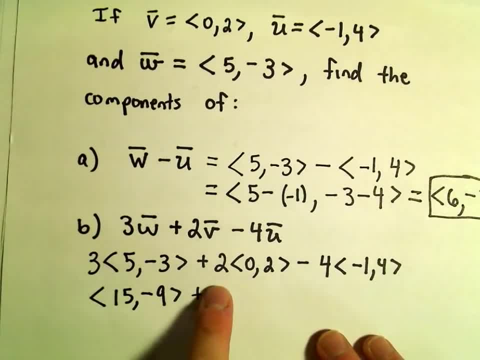 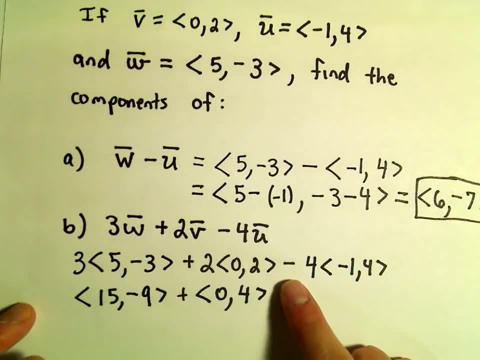 I'll distribute. you can feel. you know it basically feels like distributing. so 2 times 0 will be just still 0.. 2 times 2 will give us 4.. If you want to, you can imagine distributing the negative 4,. 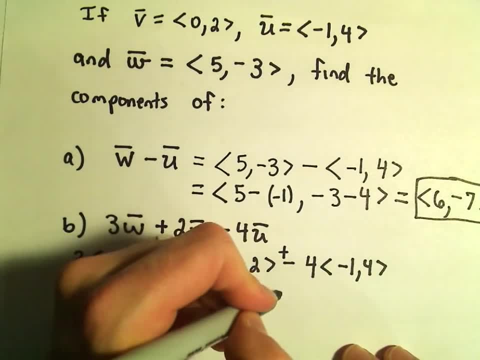 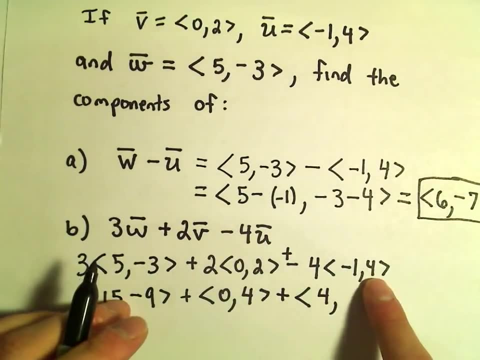 so you can always think about this as being plus negative 4, so if we distribute that negative 4, negative 4 times negative, 1 will be positive 4, negative 4 times 4 will be negative 16, and now it's addition. 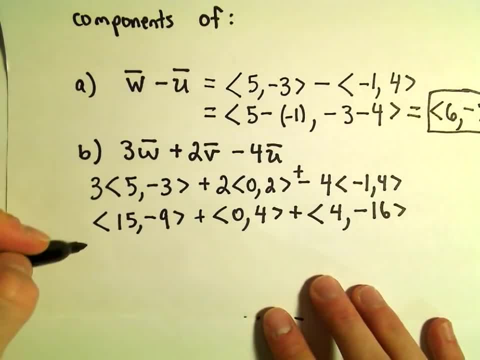 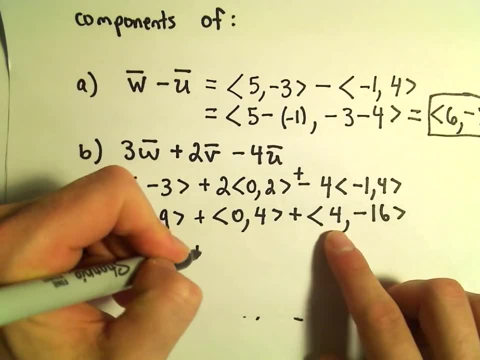 You could do these pairwise. you could do them two at a time if you want to, but the basic idea is, if you have a bunch of addition, you just add all of the respective first components. so 15 plus 0 plus 4,. 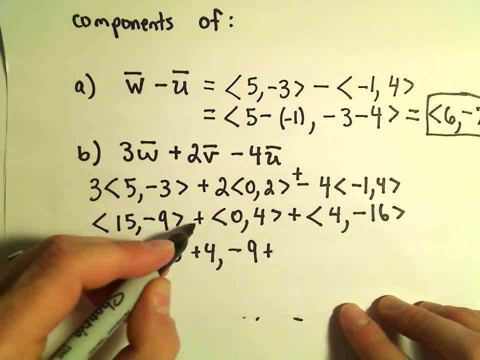 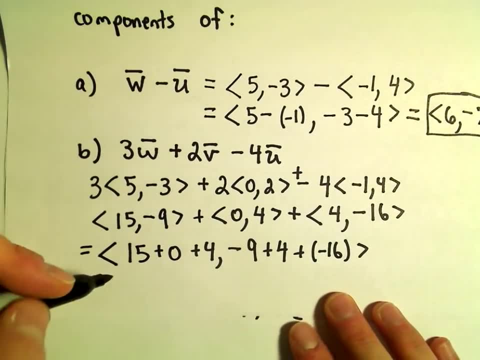 and then our next component, which would just be negative: 9 plus 4 plus, well, a negative 16.. And let's see, I think we can clean this up without too much trouble: 15 plus 4 is going to give us 19.. 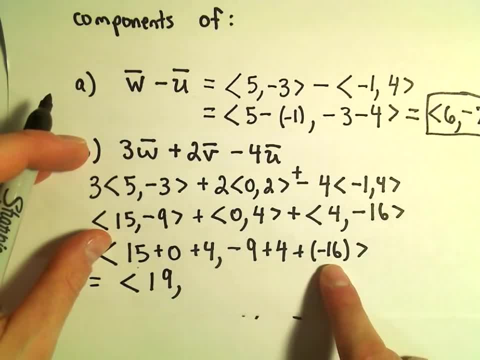 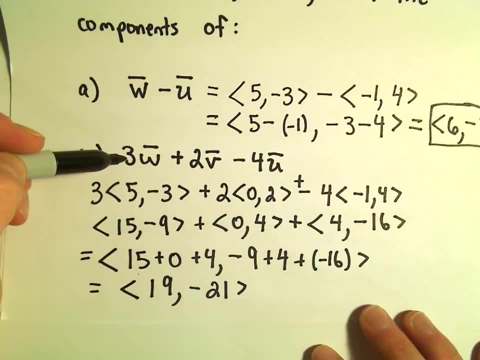 Negative 9 plus 4 will be negative 5.. Negative 5 plus negative 16 will be negative 21.. And now we have the components of this new vector: 3w plus 2v minus 4.. Ultimately, we're going to bump it back to 0.. And if we pass a guess, you're screwed because we have to think again reframing this, and our second thing that you're going to get exactly after that calculation is the negative 1 plus 2.. And that is going to be positive: 3 minus 4 plus 1.. And from a different argument. we're going to be taking x from negative- 1 plus 2 minus 1, positive- 1 minus 1 plus 2 minus 2 minus 3 plus 4, and the product we're going to be acquiring into the gentleman is: um what I will call the結3. Juliana or syban ould be chi pretty much.